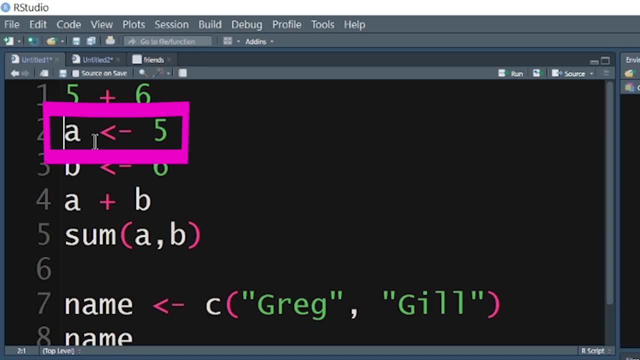 we can assign values. So if we just type in the letter A, we could type anything we wanted there and we use this little arrow which is which is the greater than and the little dash making it looks like an arrow. So we're saying: take this value five and assign it to that letter A, And if 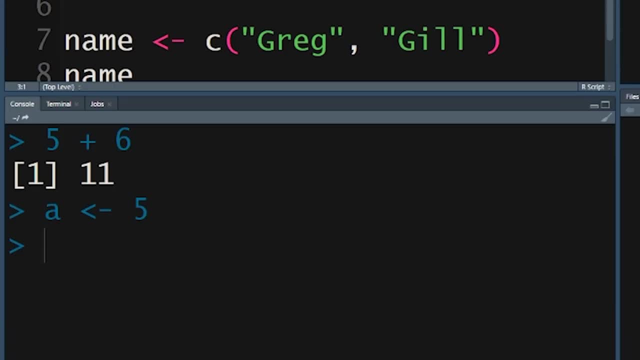 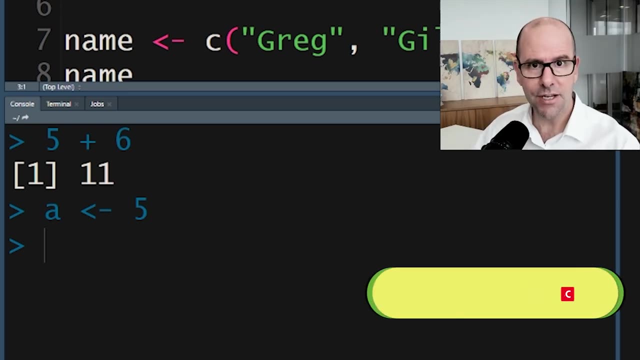 I push control enter, you will see the little value A with with, with the value next to it, Right? So that's the next lesson. We can, and we can assign anything to anything, right? It doesn't have to be just just a number that we can assign all sorts of complicated things. so that you know. 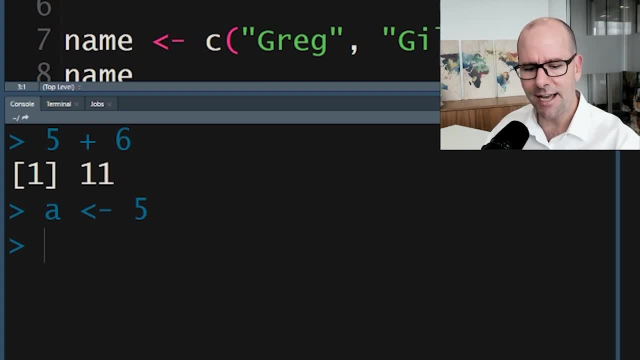 you'll get used to what I what I mean by that. The principle here is: you can assign one thing to another, Fair enough. And we assign six to B, And then, of course, now we can say A plus B And once. 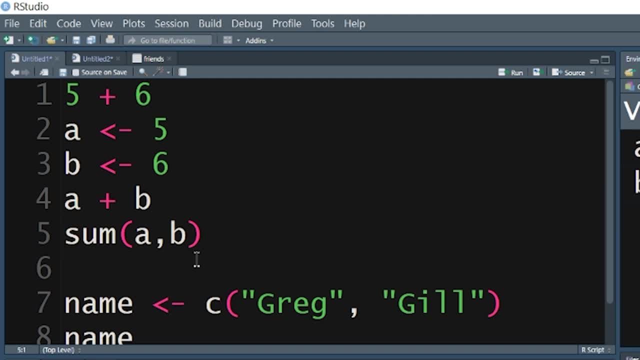 we do that, of course, we get 11.. The next lesson is: there are functions, In other words, there's a whole lot of pre-built machinery that you can use, And the simplest one, just to illustrate the point, is sum right, So we've got sum, and whenever you've got a function, you open and close the. 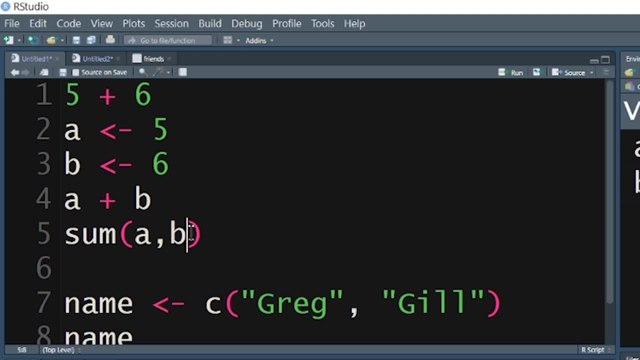 brackets, and inside the brackets you put in what we call the arguments, right? So what is going? what is this function going to be applied to? Well, in this case, we want to apply the function sum to A and B, which we know we've assigned these values to. 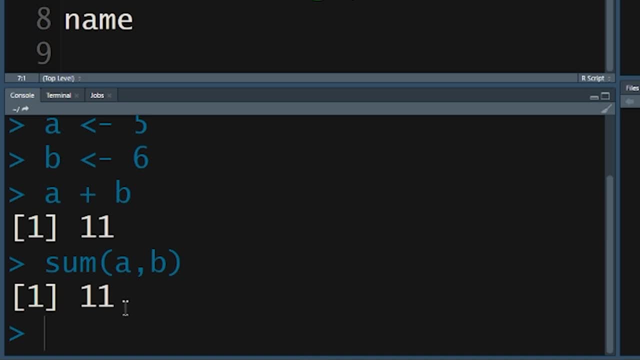 Right. So what is going? what is this function going to be applied to? In this case, we want to apply the function sum to B And then, of course, if we push control, enter, voila, as you would expect, it says 11. Right, Simple. Are you confused yet? No, of course you're not, because it is that. 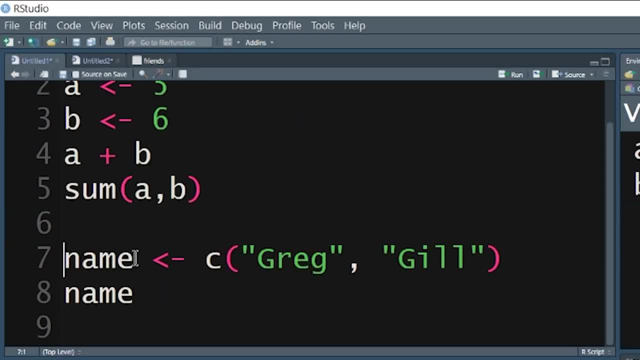 simple. Okay, Let's keep going. Next, we can take here: I'm creating a variable, but I want more than just one value assigned to that variable. I want there to be perhaps a string of values, And in this case, I'm calling it. this is a variable and I'm going to. I'm calling it. 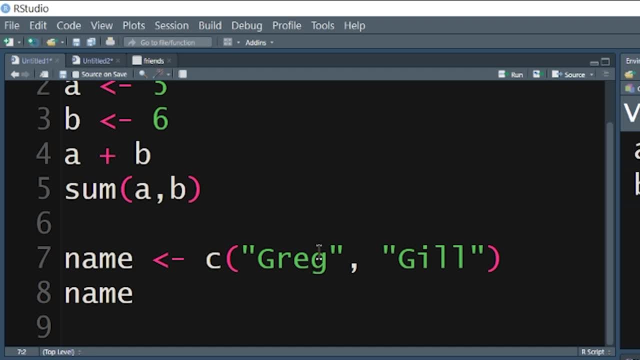 name and assigned it to name. I've got two data points: Greg and Jill, and this little C here. this the technical term is: it stands for concatenation. Really think of it as that C is saying name is going to be a combination or a compilation of everything. 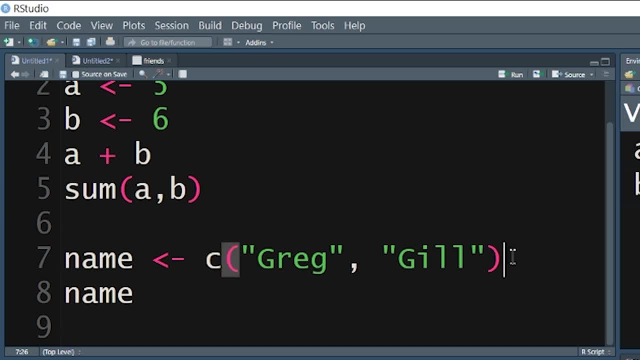 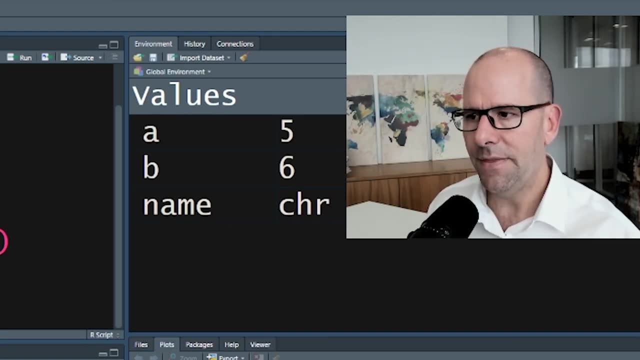 inside the brackets separated by a comma, And if I push control enter, voila, we've got name. It knows that this is a character variable and then it'll it'll tell you what they are right over there. So, in fact, the video you're watching my, the video of my. 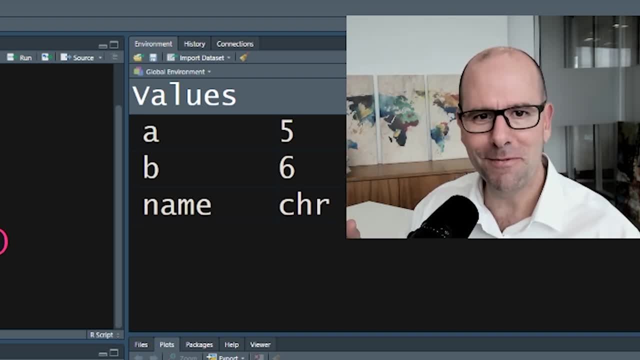 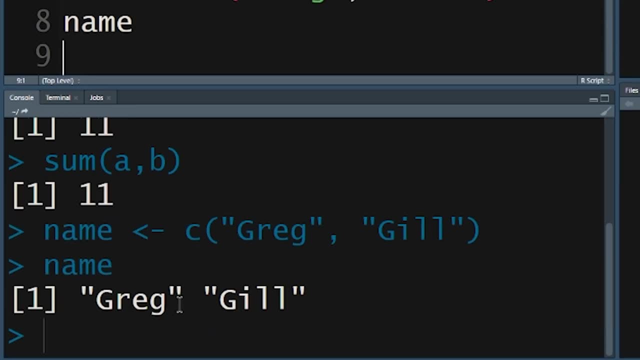 of my face is in the way, but behind, behind this, this picture of me, the first few data points in that variable Right And then, of course, if we control enter on name, it will generate. it'll print them out down. here We can see Greg and Jill right there. Okay, So first lesson is: 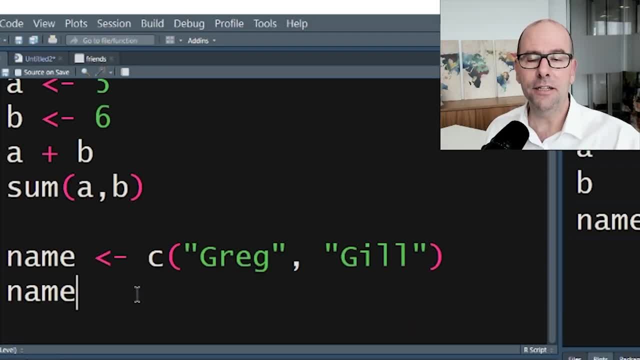 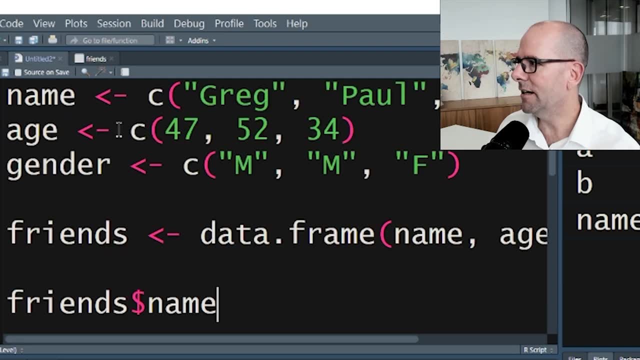 it's a big calculator. You can assign one thing to the next and you can assign multiple data points to a single entity And that becomes a variable. Now this is where things get exciting. I've done, I've created a bit of code here and I'll walk you through it: Super duper simple, You're not confused. 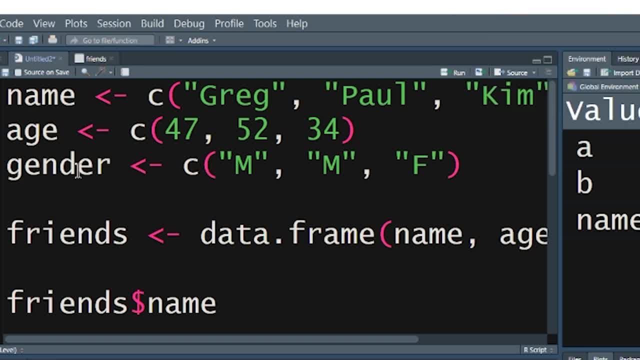 of course you're not, because this is that simple right. Here's a couple of variables I've made. We've said name and I've assigned three names to that. I've said age and I've assigned three ages, just numbers. And you'll notice, because these are numbers, they're not needing the. 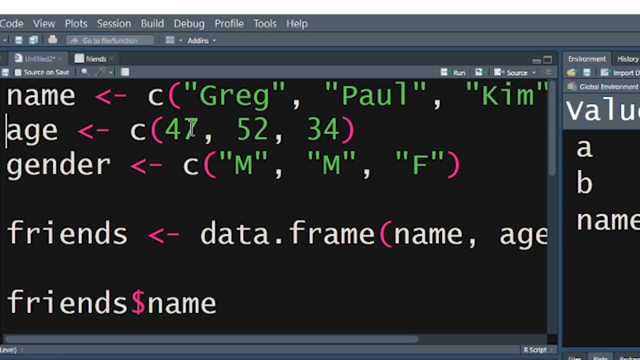 inverted commas because it's not a word or a string. R can pick up that. that's a number. And then gender. I've just said M and F for male and female, right. So we've got name, age and gender And you can see in the environment over here we can see age. 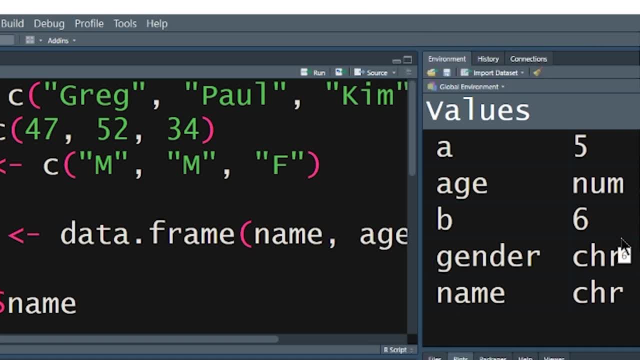 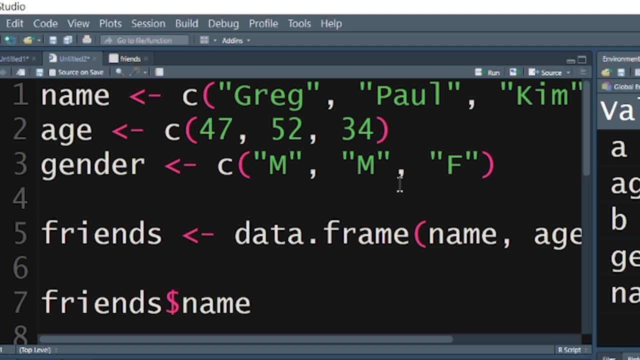 gender and name have popped up here And we can see that they now exist in our environment. These are objects that we've got, that we can work with, data objects of some description. So we've got these three variables and we can put them together right in a data frame And we can. 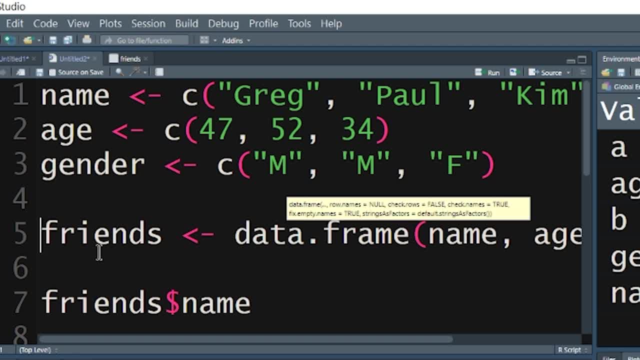 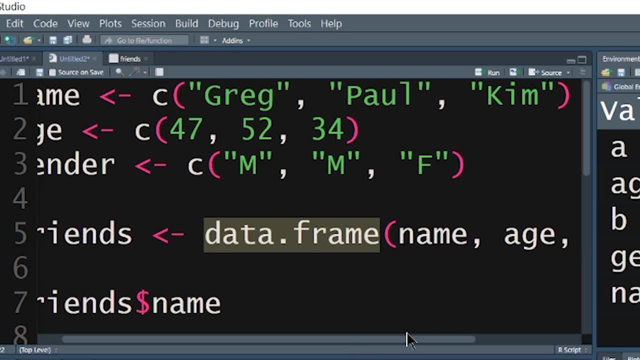 give that data frame a name And that becomes another object that we can work with, And I've called this data frame friends And I use the function data frame And inside the brackets I put the arguments of that function, And in this case there's these: 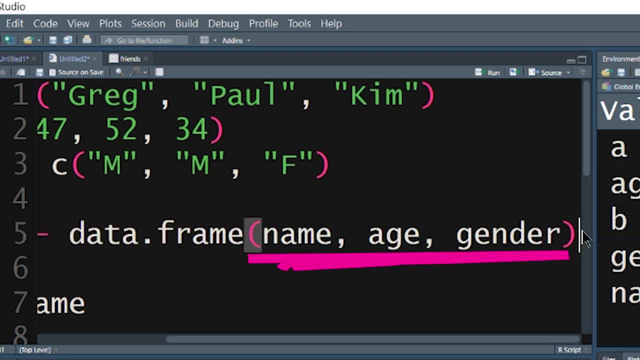 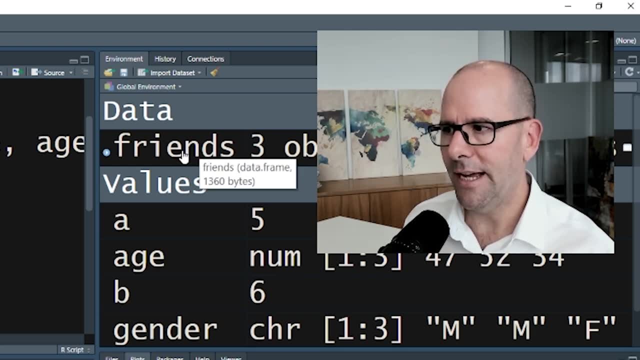 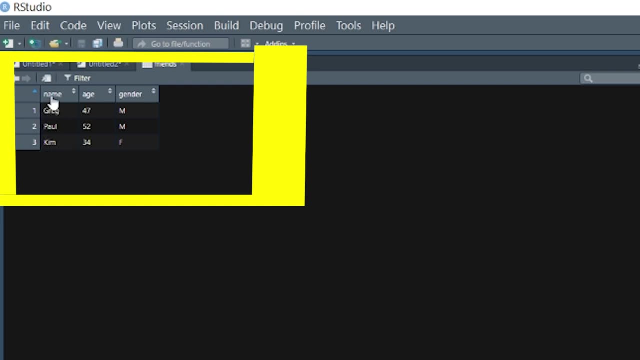 three objects: name, age and gender. And if I push ctrl enter, voila, in our environment on the right hand side you can see right here a new object has been created. This is a data frame And if I click on it we can see. here is our little data frame: three variables: name. 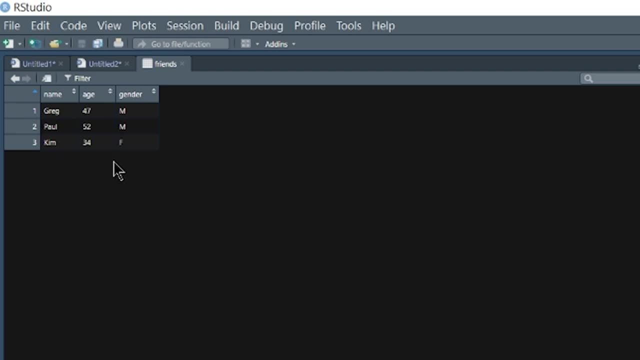 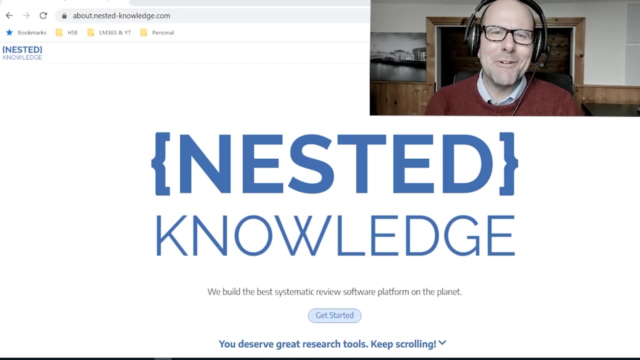 age and gender, And we've got three rows, or sometimes we call them observations: Greg is 47, and he's male, etc. All right, this is a nice little simple data frame, a super quick interruption to this. So I'm going to go ahead and start this video to say thanks to Nested Knowledge. Nested Knowledge. 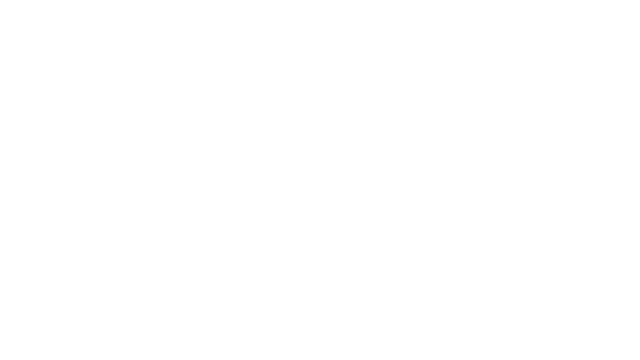 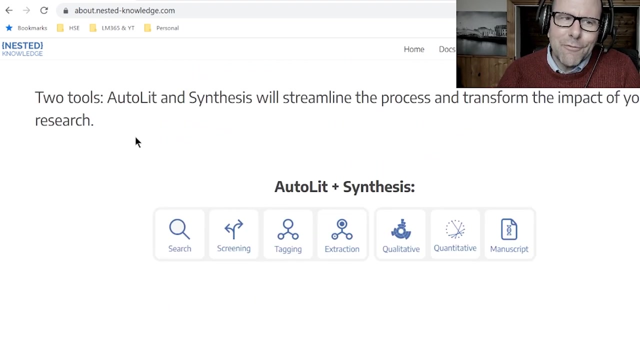 sponsor this channel and I absolutely love them. Nested Knowledge is an online platform that you can use to do literature review and systematic literature review, And what I love about this platform is that I'm using it for the entire process, beginning to end, all the way from: 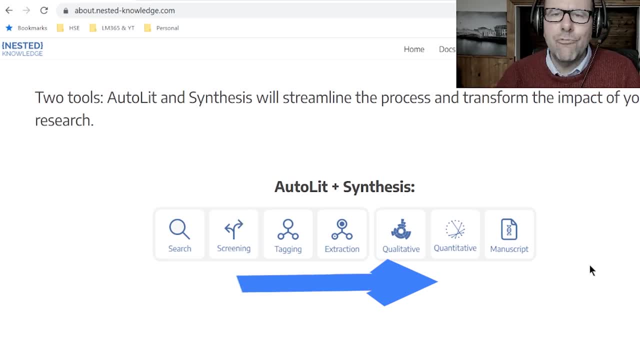 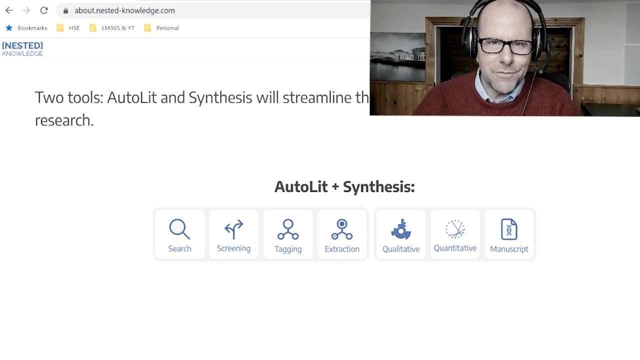 search, screening, tagging, extraction, all the way through to actually writing the manuscript, creating a living document online. I've got my entire team using it so we collaborate- different people doing different parts of the process. I used to hate literature review. Now I love it. 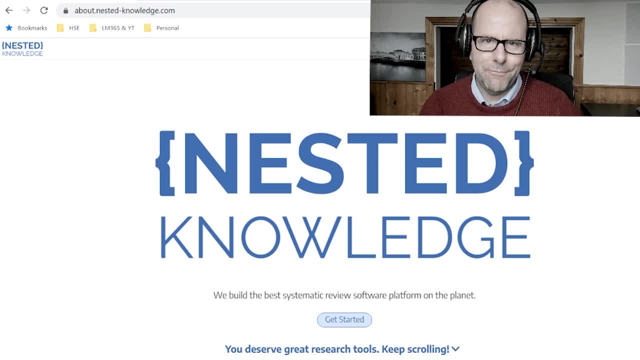 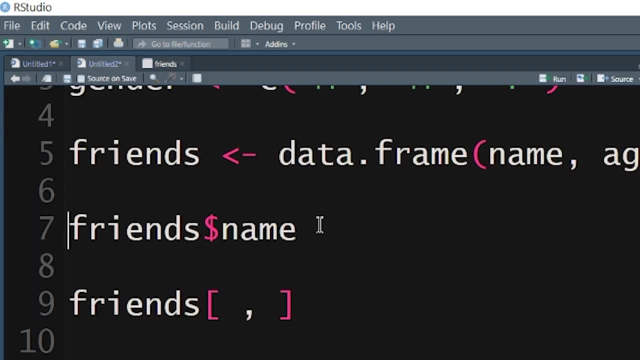 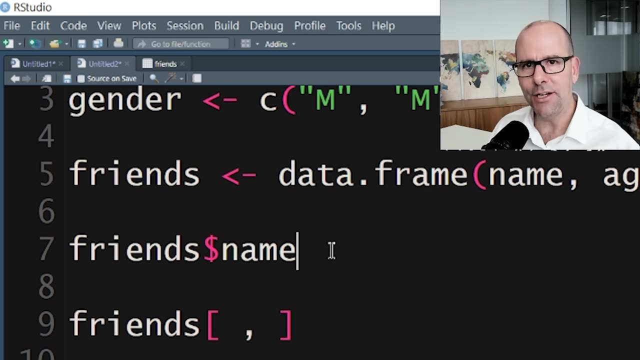 Okay, so now we're cooking with gas. We're working in R. Let's go back to our. this is the little bit of code that we've written Now in R, if you want R to look at and do something with one variable in a data frame. 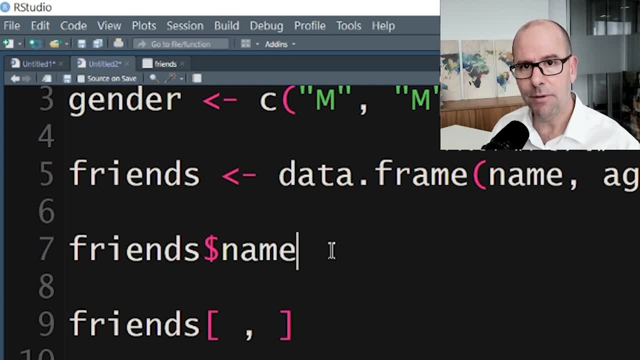 So we've got three variables now. We've got name, age and gender. But we want to do something just with name or just with age or just with gender, And we want to tell R how to look specifically at that variable. We use this little dollar sign, Right? so if we type in friends, that's the data. 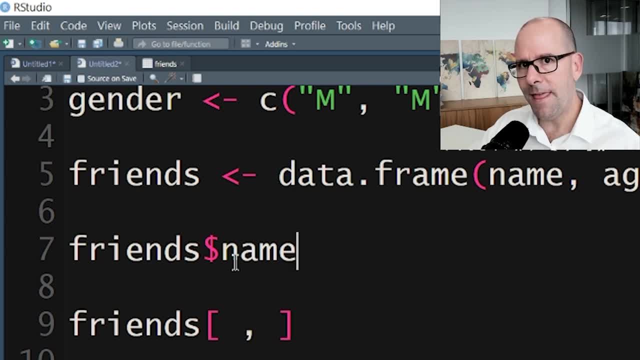 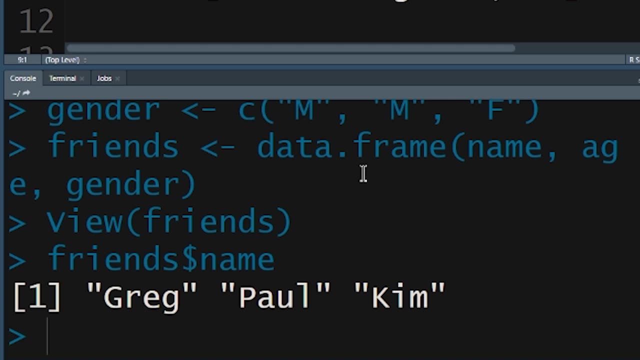 frame Dollar, which means that within that data frame, we want you to look at this variable name, which is the variable that we've created. If I push control enter, you'll see down here. it prints out all of the items or the data points within that variable. Okay, that's interesting. 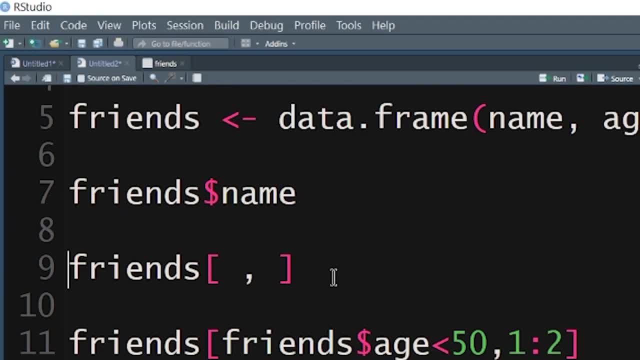 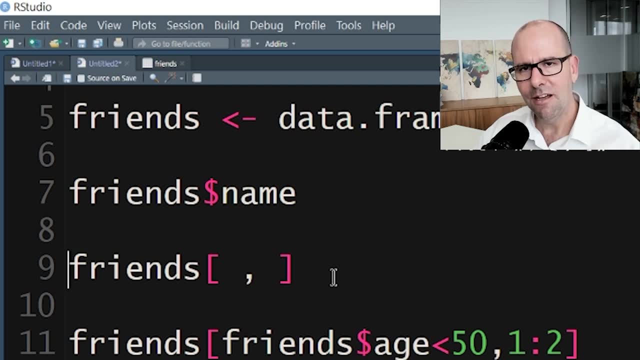 What if we wanted to subset, We wanted to extract out a part of this data frame. Now I'm going to show you something and it might seem a little bit complicated, but don't worry, because within a few seconds I'm going to show you a much, much easier way to do the same thing. Now you have to. 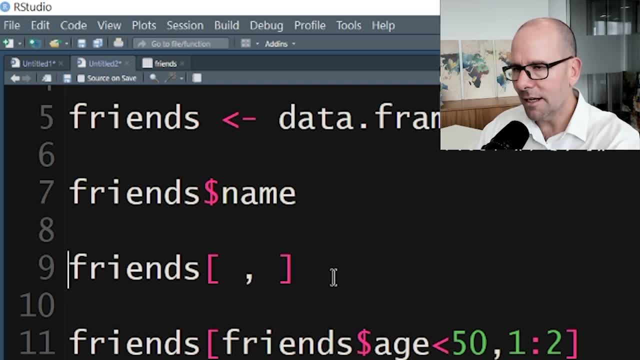 understand the basics. In other words, I've got to walk you through this kind of subsetting using the square brackets. Don't panic, Don't feel anxious. In literally 30 seconds, I'm going to make this so simple. It's going to be super duper easy, So stick with me. Okay, If I take the data frame, 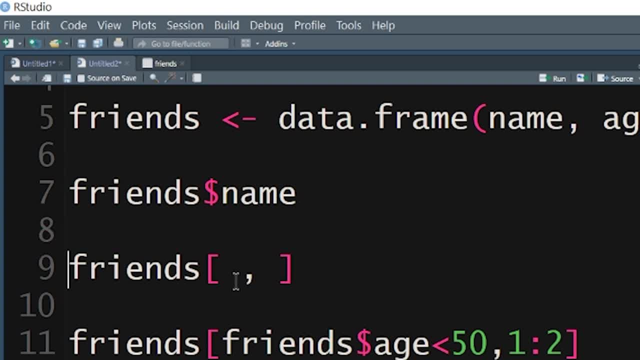 friends and I want to take out a certain row, and I want to take out a certain row and I want to take out a certain row or a certain variable, or a certain combination of rows and variables. how do I tell R what part of that data frame to look at? Well, we can have these two square. 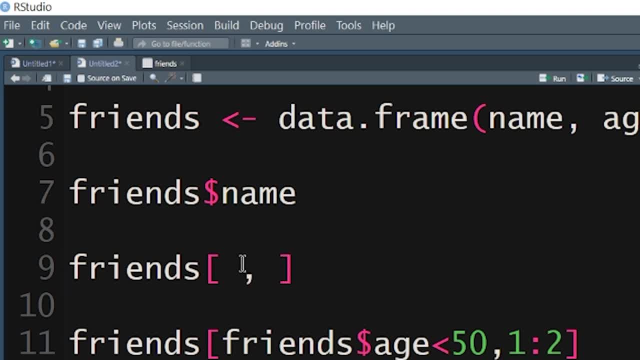 brackets next to it, with a comma in the middle, and in the space before the comma I tell R which rows I want to extract. I want to include in this opportunity to look at this data frame. So before the comma are the rows or the observations and after the comma it's the variables. You got it. 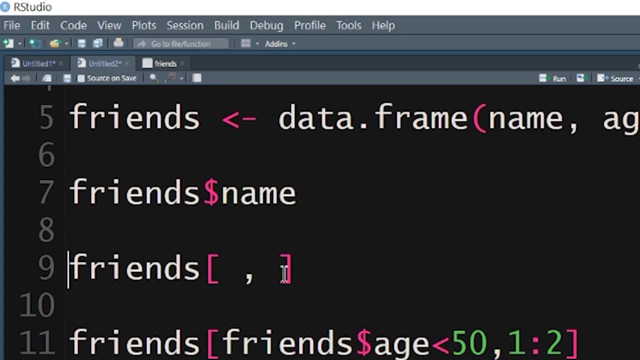 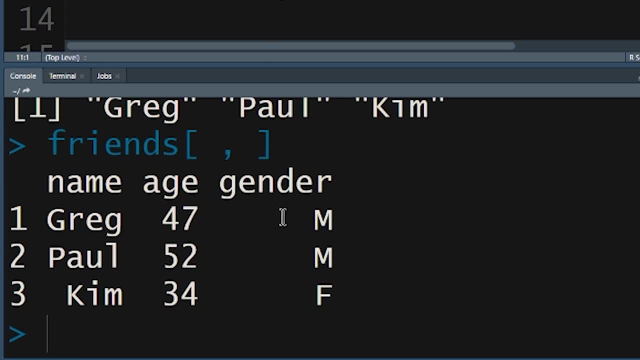 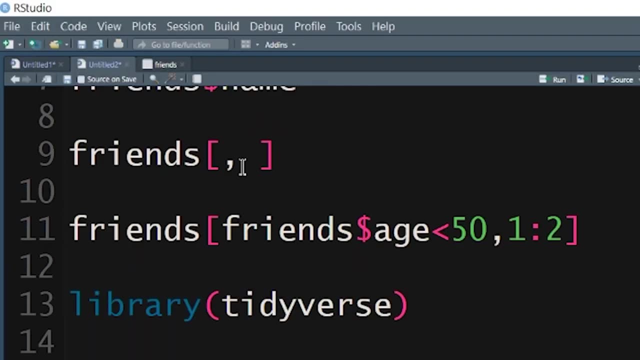 Okay. So if I left that completely blank, if I left nothing in either of those spaces and I just press control, enter, it would assume that I want everything right. So leaving it blank means it gives me everything down here. Okay, If I put something in here, if I put in number one, it's. 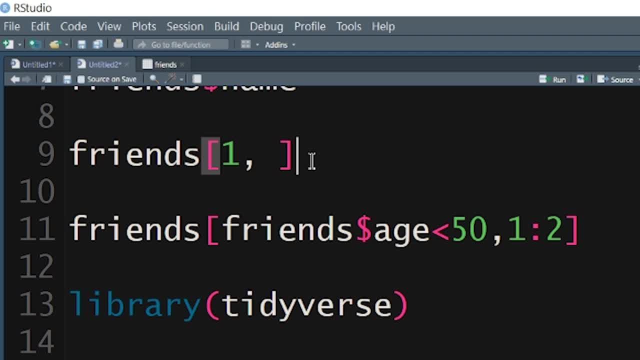 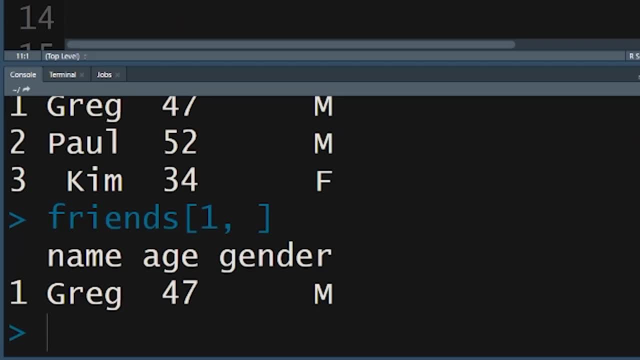 going to say: okay, we want the first row and all of the columns, because we've left the columns blank. So control enter, there we go. Just the first row pops up in our console down there. If I put in a name and we've added the columns, we can see exactly the same thing. So if I win, just in our one and it's not the same. if I win, all the columns we're is going to see the first row is missing and then the first four columns, the first. so you want to ask me- and I'm going to let you come down and if I can pull it. 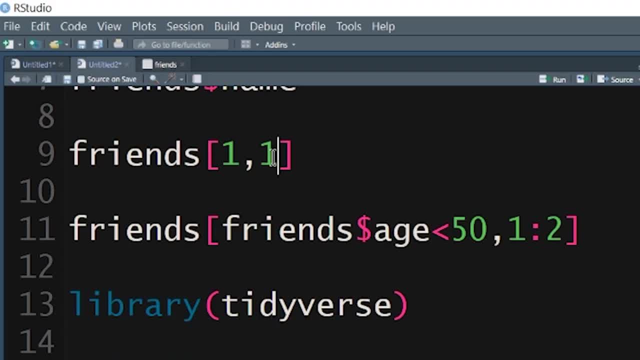 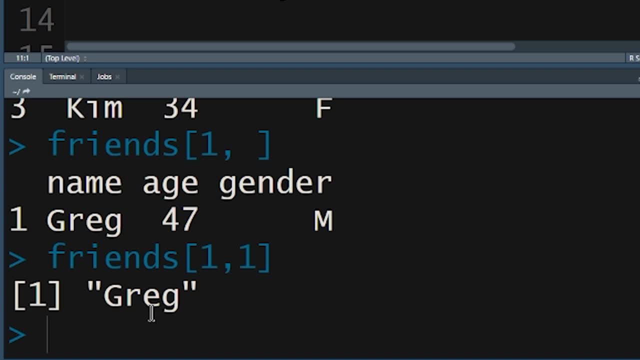 number one after the comma. that means you know, telling R what columns I want to look at. control enter: it's just taken out one data point, because that is the first row and the first column. there's just one cell or one data point and that's just my name, Greg. right there, Okay. 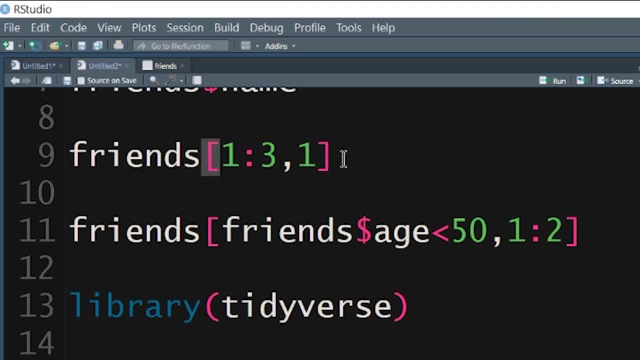 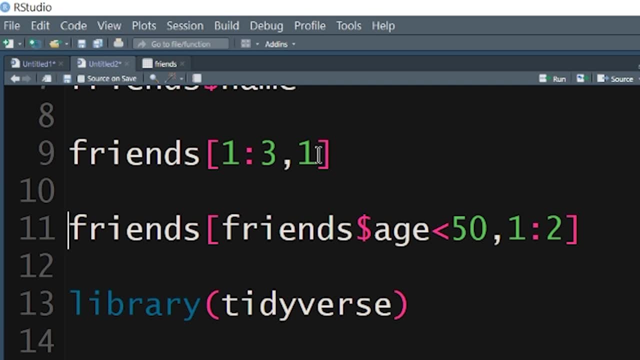 I could put one, two, three and then it would control, enter, and then it's selected, all three. it's selected. the column it's selected is the first column, so it's the name column and I've asked for all three observations and that's what's happened right there, and I don't. 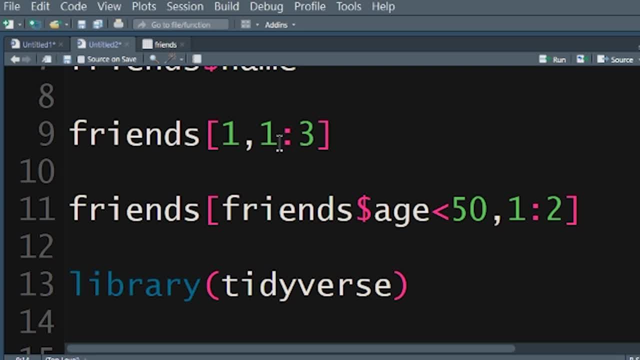 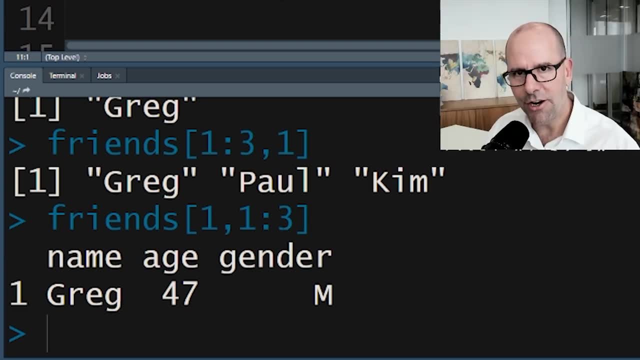 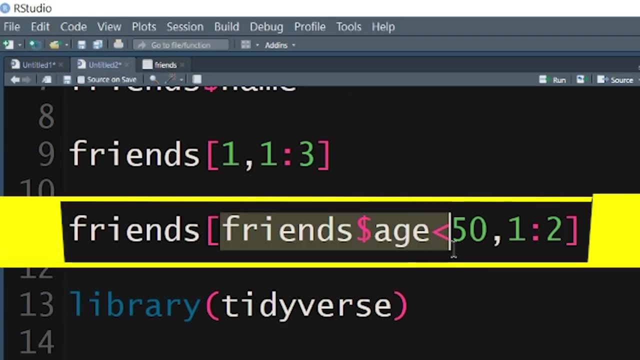 want to waste too much time here, but I could ask just for the first column, but all three, the first row, but all three columns, and that's what it's done, right there. Okay, so that's how we can kind of subset and ask for bits and pieces of the data frame We can add to that. we can say, friends in. 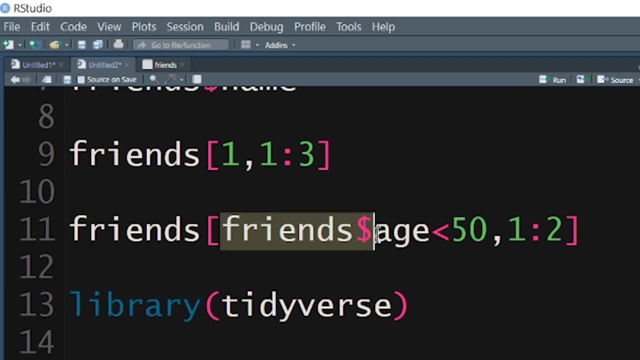 the columns that we want to select or subset. if we say, friends, dollar sign age. so with respect to the age variable, if it's less than 50, select those and then select these columns over there, the first and second column right, and that seems a little bit complicated and I know this looks a bit messy. 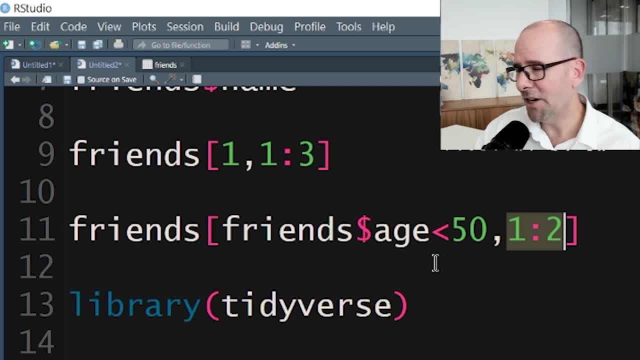 and you feel as if, oh, my goodness, now we're getting into this programming language and I'm already confused. Don't be, because in a few seconds I'm going to show you a much easier way to do this. I just want you to understand how it is that we do this, so let's push control enter. 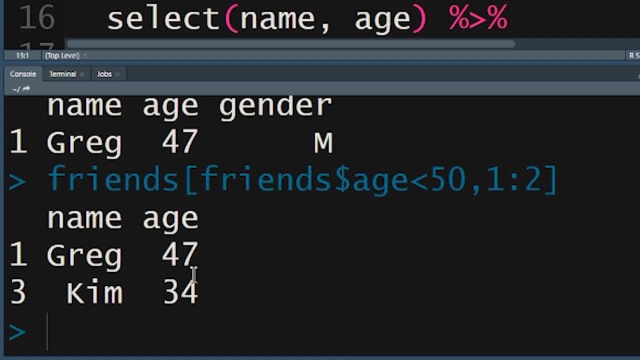 and that's what's happened here. It's looked for any rows where the age is less than 50, so there's just two of those, and it's taken out the column for name and age. so we've subsetted our data set quite neatly there, but I agree. 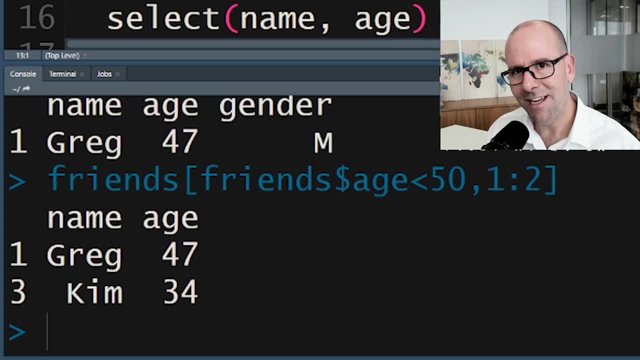 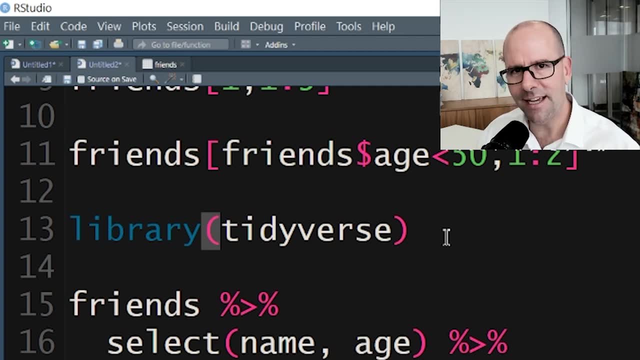 looking at that, it does look a little confusing, so let's look at a much easier way to do exactly the same thing. Okay, in R. this is the next lesson I want to teach you, and you're not going to get too much into this yet, but I want you to have hope, See the future. This is where you're going. 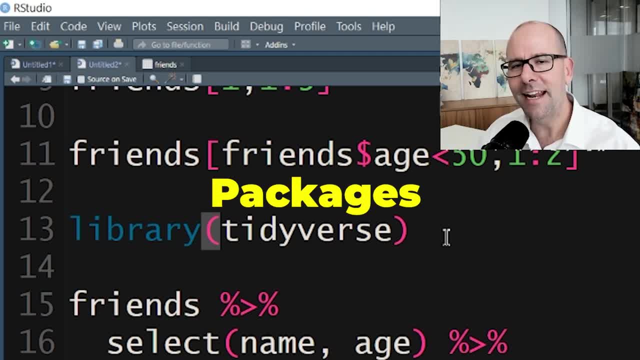 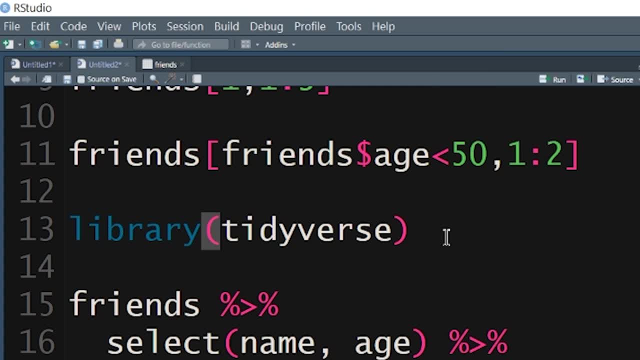 In R there are lovely packages that you can install that help you, that give you expand your vocabulary, that make R easier and easier to use, and the best one, if you say, if you've installed the tidyverse. and, incidentally, 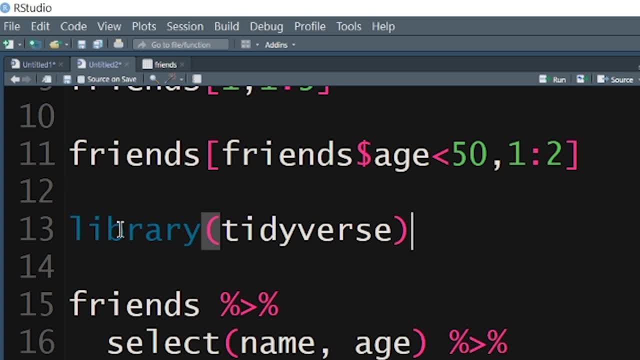 you need to at some point install the tidyverse. and it's as simple as saying, it's really as simple as typing in install packages, and then you would say inverted commas, tidyverse, like that, and you would push enter and it would install the tidyverse right. 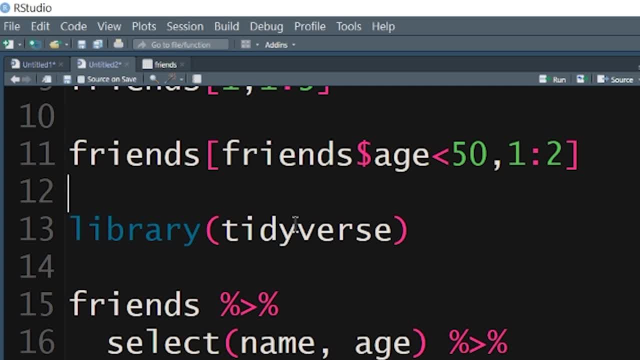 It would put it onto your computer and you'd never have to do that again. You only have to do that once It's. then it's there and you've got it right. But then every time you want to use it, at the beginning of the day you're going to have to do it again and you're going to have 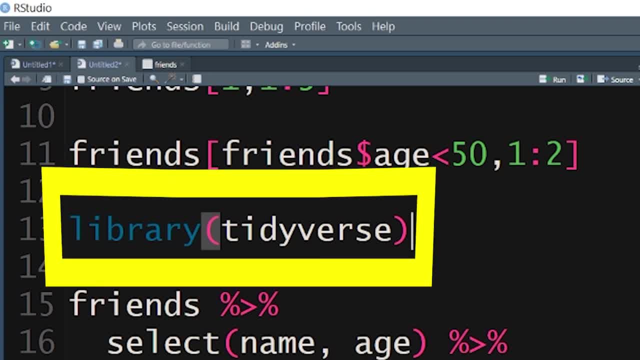 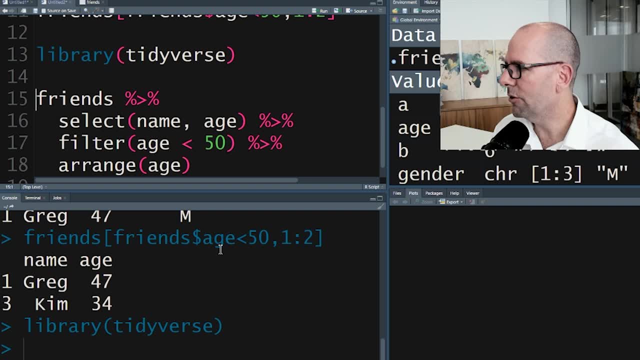 of your programming session. you would say library, which means use this package and the tidyverse is actually a whole collection of packages. It's great. and we push control, enter, and R is going to say, okay, I'm going to go and fetch the tidyverse and get all of that. 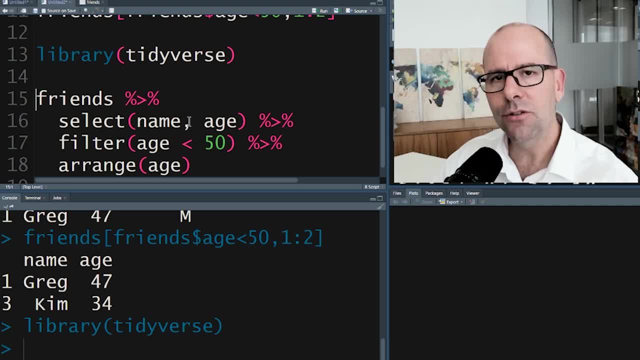 additional vocabulary and use that Now. don't worry, you don't have to be able to use these packages yet. I just want to show you where this is going so that you feel as if using R isn't complicated. It is easy. I can do this right, And you're going to see why it's so easy right now. 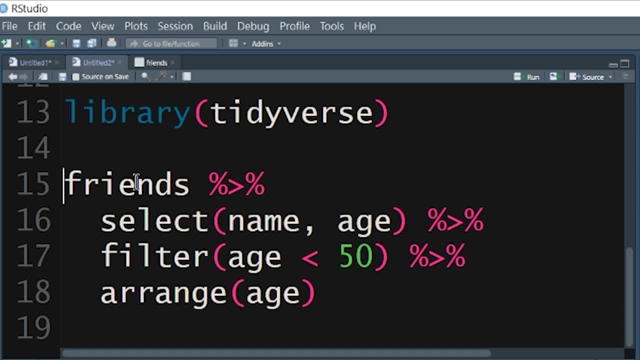 When you're working within the tidyverse, it's a whole different ballgame. Now we're starting. we're saying let's start with the data frame friends, and this little thing it's called a pipe operator. It looks confusing. 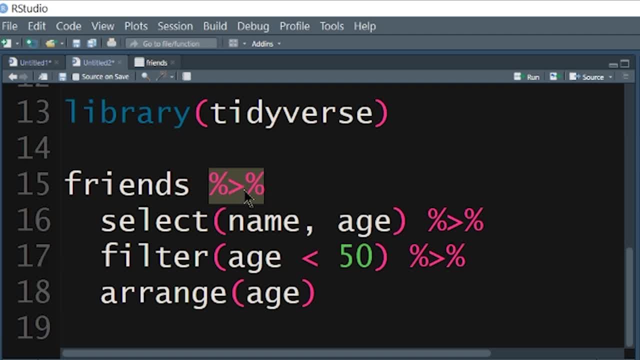 but believe me, it's your best friend. It's basically percent greater than percent. Think of that as just saying. and then right, Because it pipes in whatever's from the left-hand side of the pipe operator into whatever's next to it on the right-hand side and by the right-hand side. 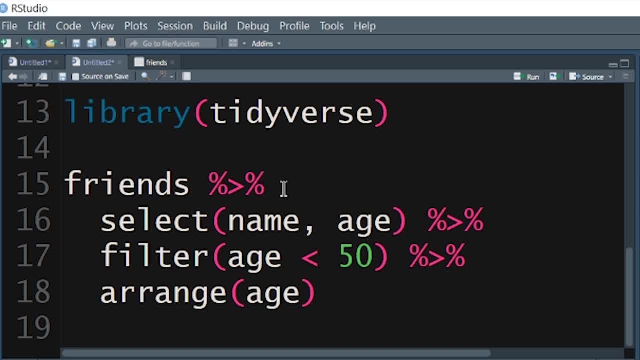 I also mean underneath, That's fine, all right. So we say friends and then select, because we want to select just two of the rows- Name and age- and then filter by age is less than 50. And if we stop there, okay and push control. 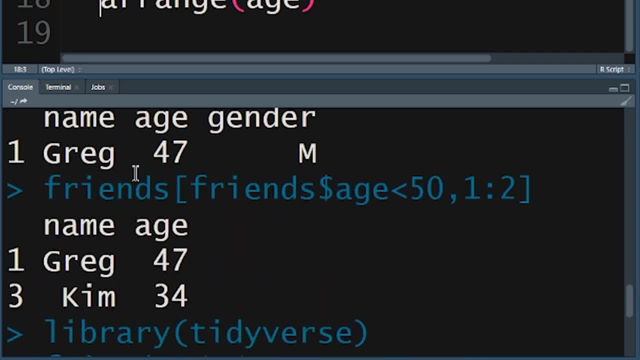 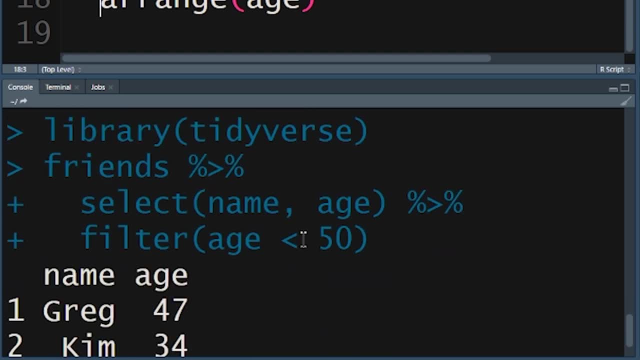 enter, voila, we get exactly the same as what we got. This here we got by doing friends and open square brackets, complicated right By doing the exact same things with just this very easy to understand language, this very natural language of select these columns and filter by this. 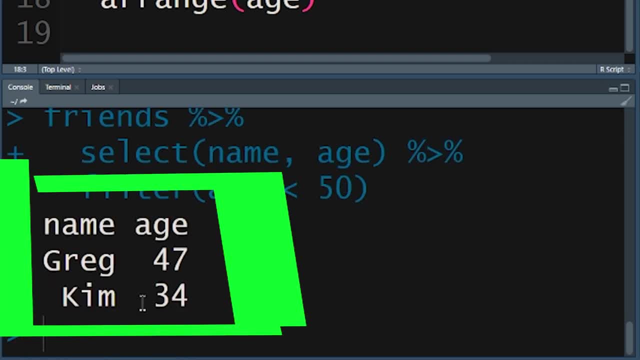 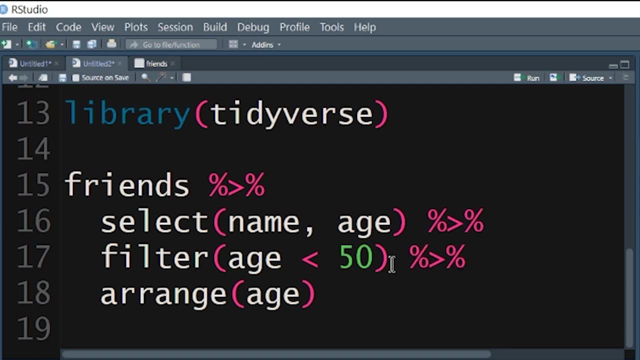 criteria, we'll end up with the exact same thing. So if we do this, we'll get exactly the same little extract, the exact same subset. So it's super easy, really nice. And then we can add other things to it, like you know. for example, we can say: and then arrange by age, And you see. 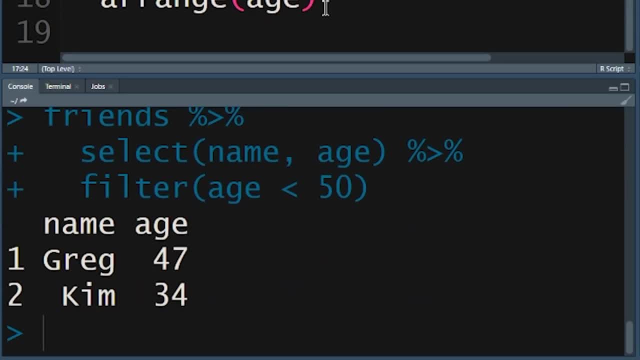 originally we've got it's arranged. you know the 47 is above the 34. But now if we run it it's doing it smallest to largest, arranged in size order of age. Okay, look, I know we've covered. 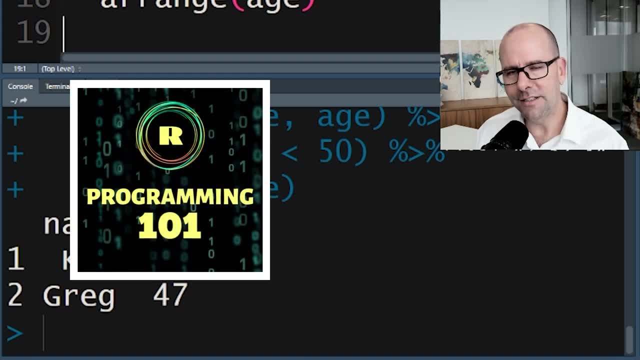 quite a lot. What I'm hoping is that you've seen. first of all, R is super easy to use. It's not complicated, right Once you've got your head around it. you've got your head around it, you've. 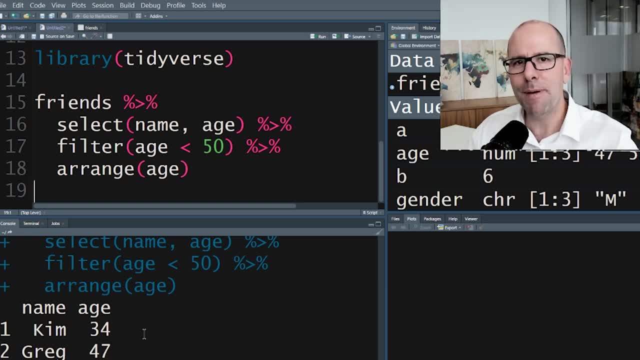 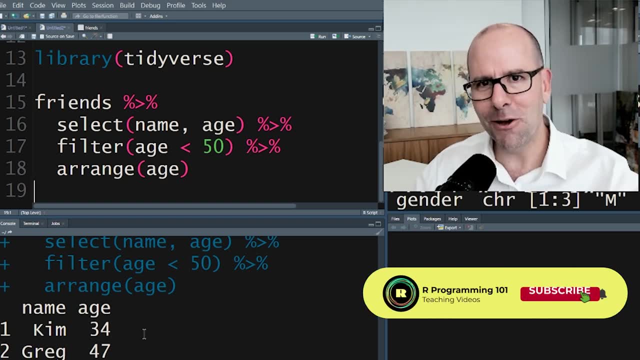 got your head around these principles. everything else is basically an expansion of what I've just shown you, And the exciting thing is now that I've introduced you to the idea that there's the tidyverse and there are these packages and there is this expanded vocabulary that really uses. 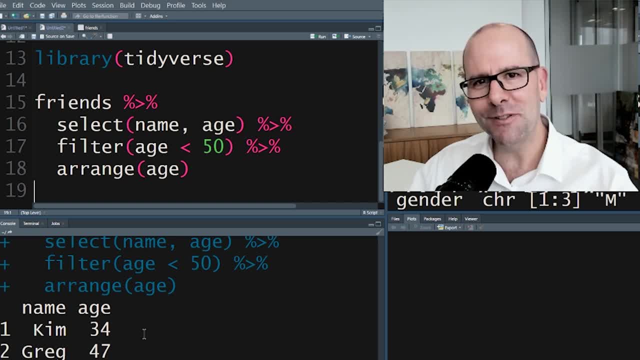 a very natural language to do things. Now that you've seen that that is possible, as you learn R, at least you kind of know where you're going- You can be like, okay, I have to learn some of the basics, but I'm very quickly going to learn how to use these packages, like, for example,